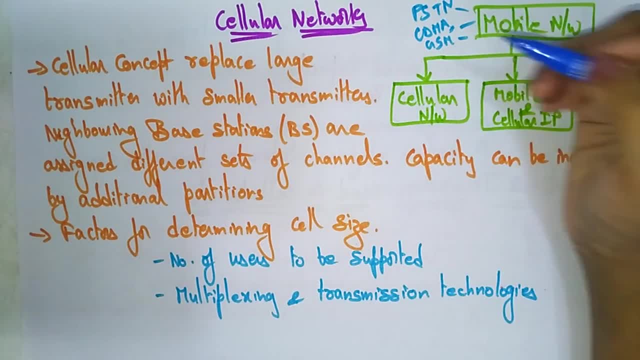 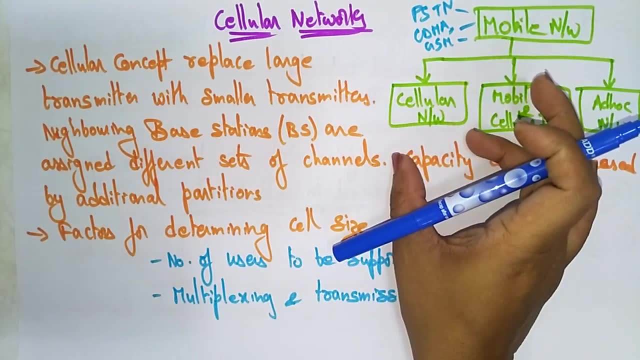 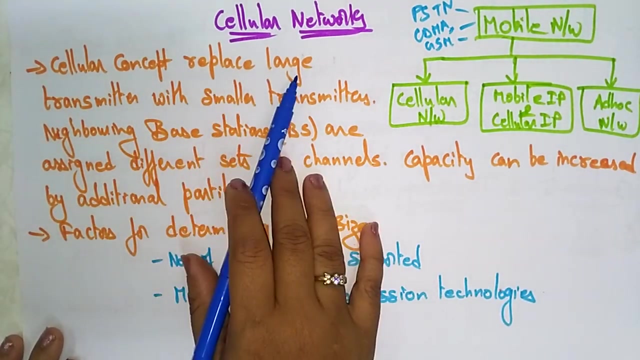 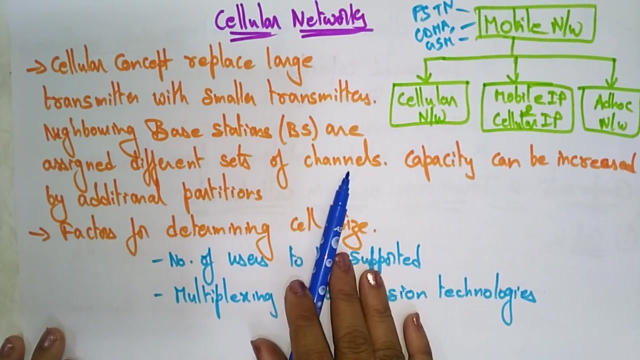 Okay, And the ad-hoc networks is the temporary networks. These are all the mobile networks. Then what about the cellular networks? The mobile network consisting of the cellular networks, mobile IP and cellular IP and ad-hoc networks will be there. Now let's see The cellular concepts: replace the larger transmitter with the smaller transmitters, The neighboring base stations or the assigned different sets of channels. Okay, The capacity can be increased by additional partition. So what it means? 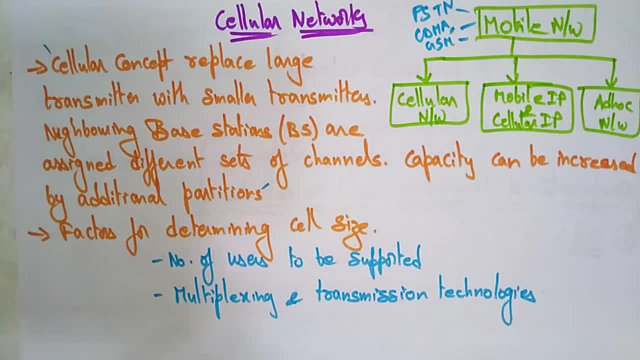 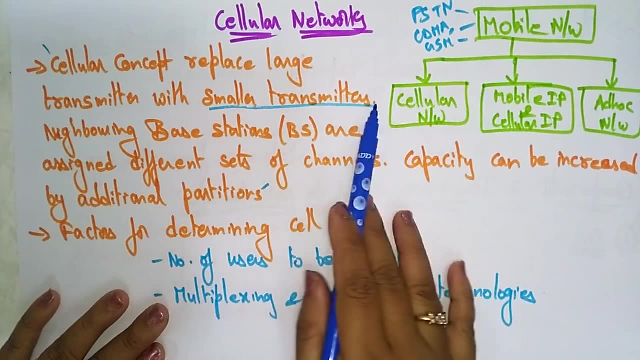 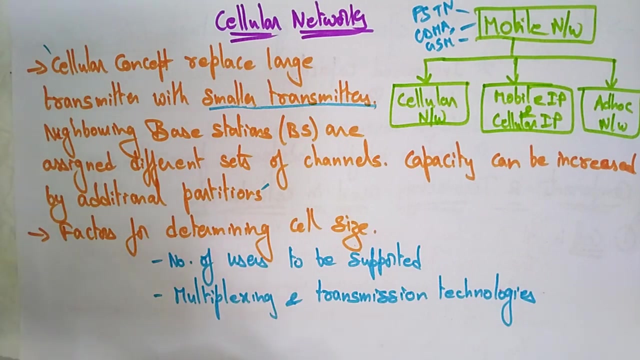 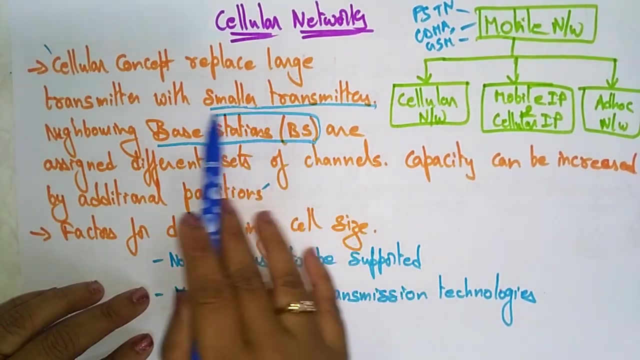 What they are saying. What is that cellular concept? The main thing we are using the cellular concept is, rather than using the larger transmitter, it will be replaced with the smaller transmitters. Okay, If your mobile is having the smaller transmitters, how can it receive the signals when we are from moving from one place to another place? Okay, With the help of the neighboring base stations, I'll explain that, this concept about base station in this video only. Okay, Don't confuse. 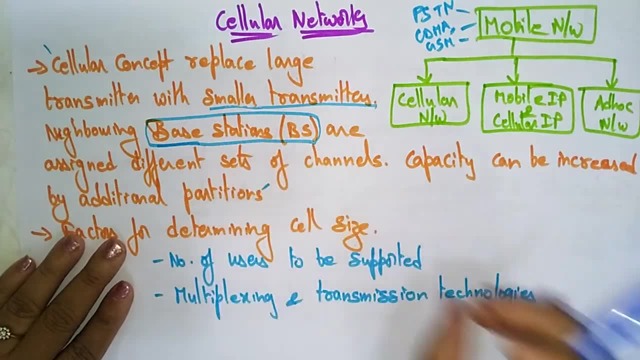 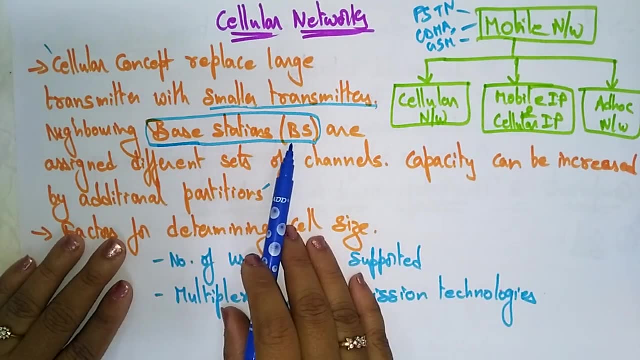 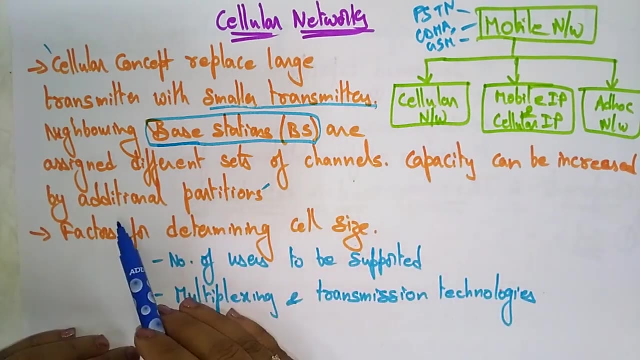 Actually, the cellular concept will replace the larger transmitter with the smaller transmitters in your mobile, which helps. even though it is a smaller transmitting, because of the base stations that are assigned different set of channels, you can receive the signals. Capacity can be increased by additional partitions. If you want, you can add additional partitions to different base stations. then the capacity can be increased. Here the factors for a cell will be provided. 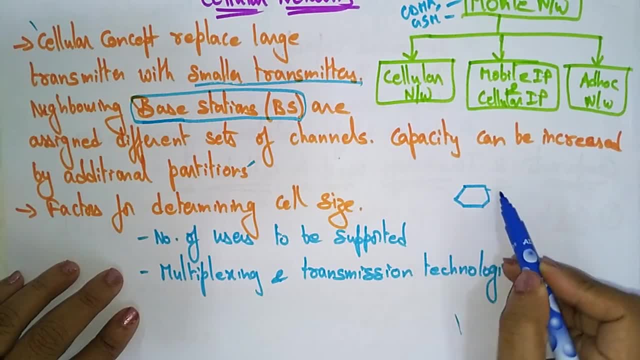 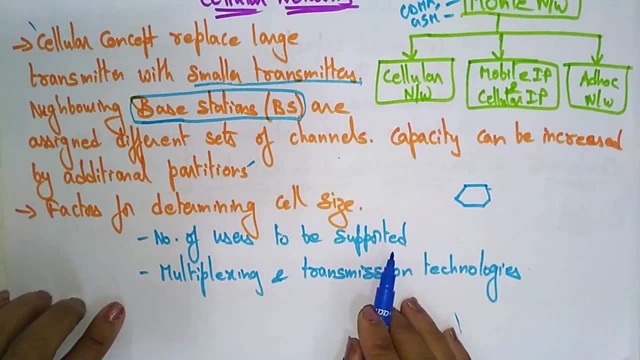 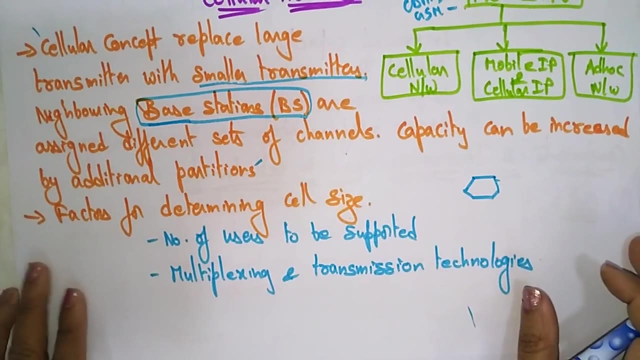 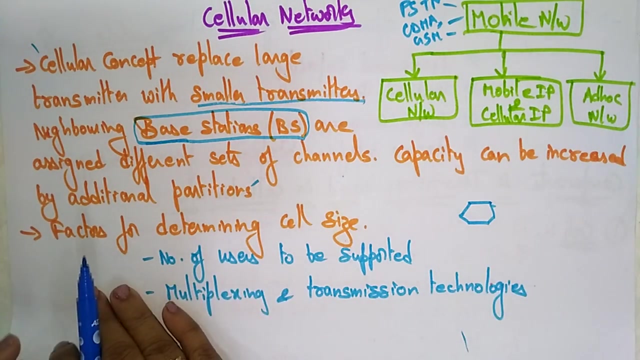 Okay, A cell will be, let's say, just represented in a hexagonal, So that I'll explain. Don't confuse: Factors for determining the cell size is the number of users to be supported and multiplexing and transmission technology. Okay, Actually, whenever you are asked about what is a cellular network, it is just a cellular concept: replaces a larger transmitter with a smaller transmitter and neighboring base stations will be there that are assigned to different set of channels. 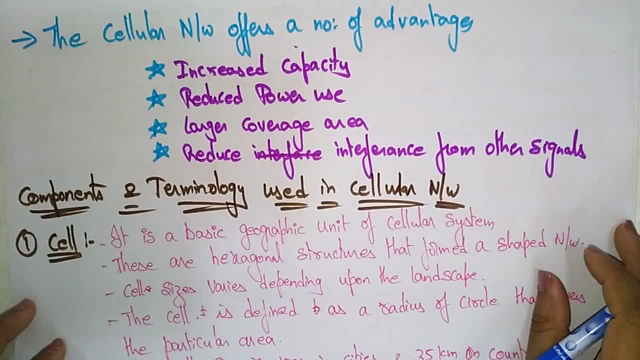 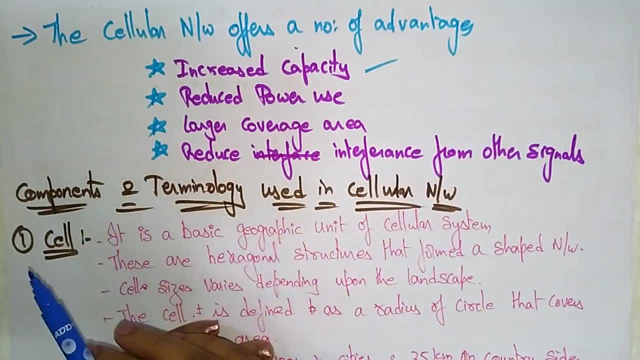 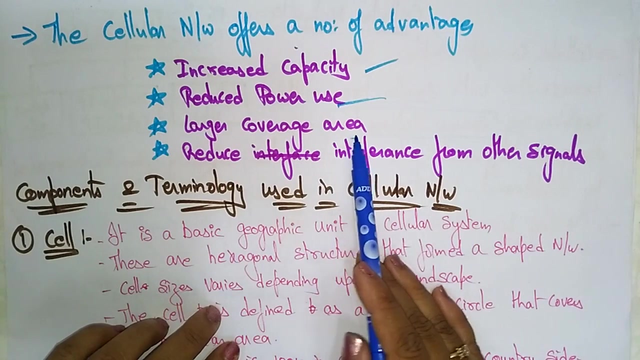 Now let's see the concept. The cellular network offers a number of advantages. What are the advantages Why we are using the cellular network? It increases the capacity. How can it increase the capacity? You can add so many base stations to each and every cell. Okay, The neighboring cells you can add, and the capacity can be increased And reduce the power use. also, Large coverage area will be there. Reduce interference from other signals. 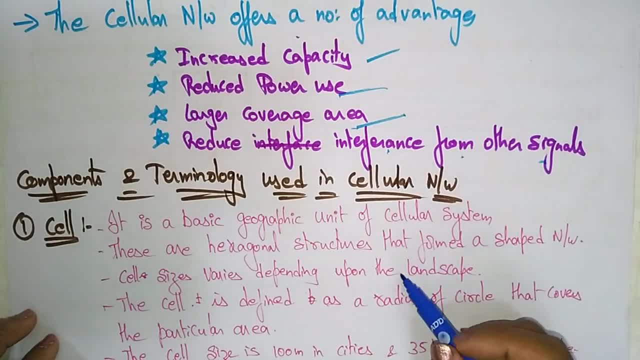 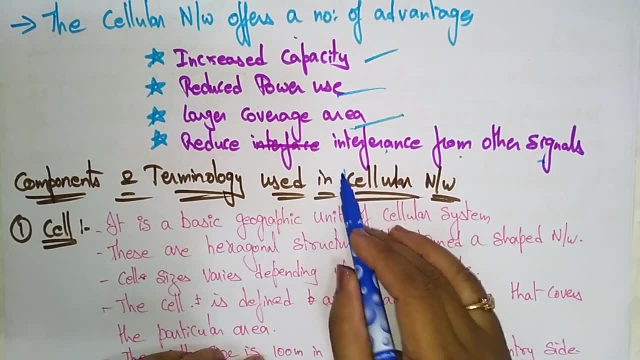 Now let us see the components and the terminals. Now, what type of components and what type of terminology is used in the cellular network. So what does this exactly? What type of components and what type of terminology that we use in the cellular network. We have to be seen. 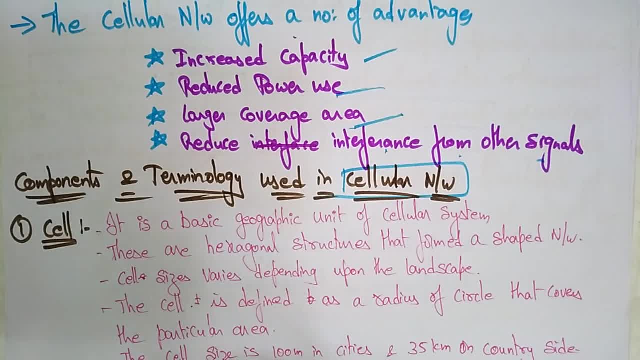 Okay, So I already said the mobile computing means it's not the external And whatever the services that you are having, that is, the networks that you are using, so how that networks will be connecting to your device that you have to learn in this mobile computing. 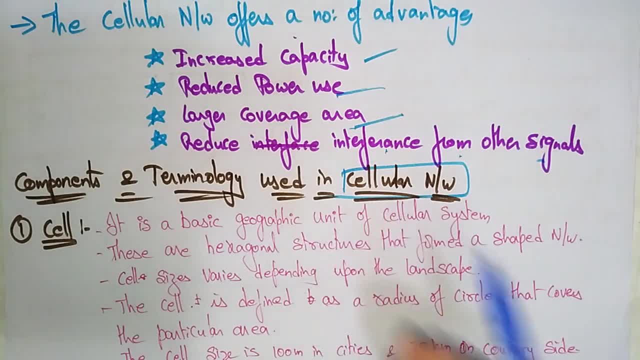 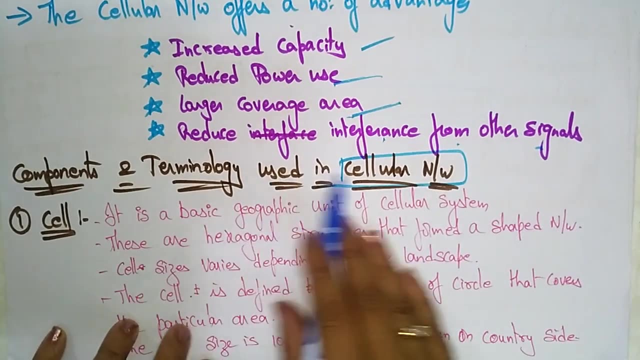 Okay, So if it is a wireless network, the CDMA technology, GSM technology, GPRS technology, wireless local loop technology, ad-hoc networks- okay, all these are the different components that are present in the cellular network. Now let's see what are the components and terminologies used in cellular network. 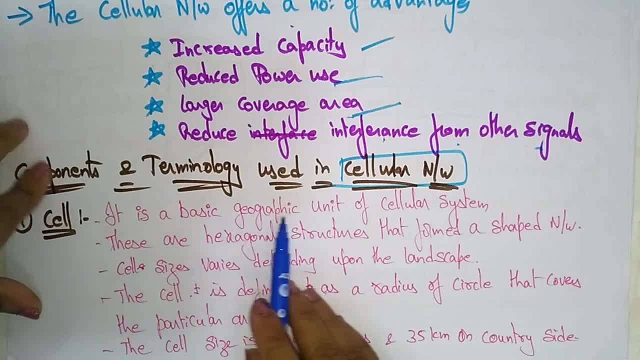 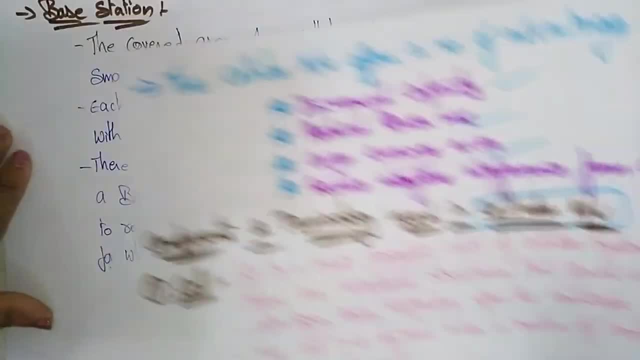 A cell will be there. a cell, It is a basic geographic unit of cellular system. A cellular system is nothing, but I will just show you. the cellular system is just represented like this: It is in the hexagonal. let me write this: 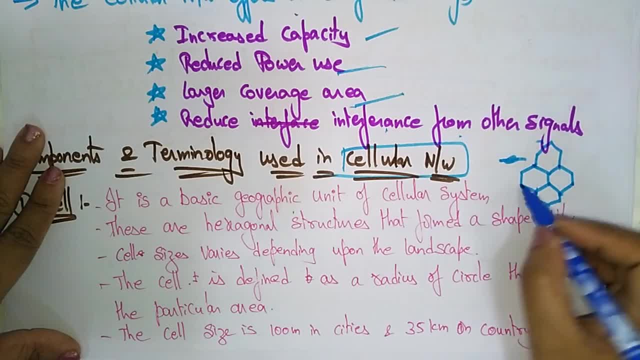 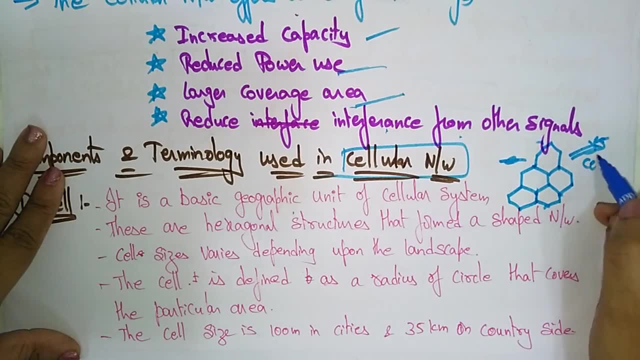 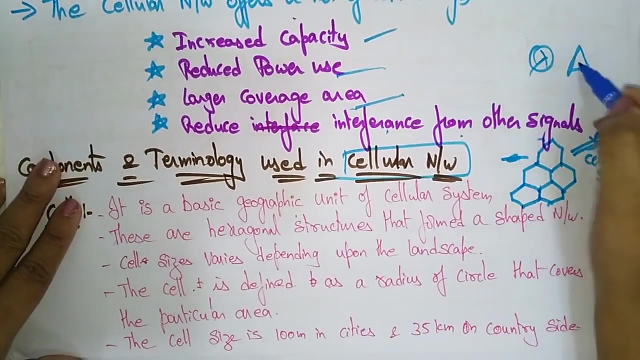 Okay, it is represented like this. the hexagonal shapes This complete structure. you call it as a cellular net system. Okay, cellular system. Why, I am taking Only the hexagonal, not the circle and not the triangle. okay, and not the rectangle. 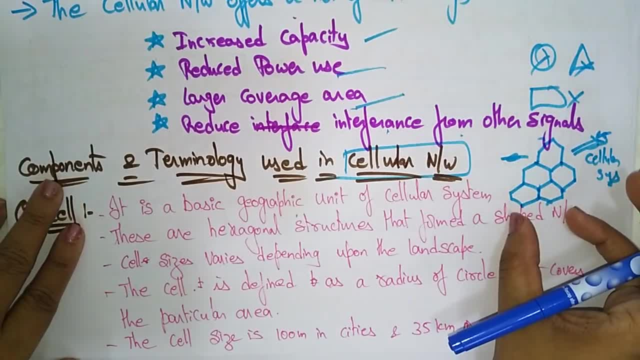 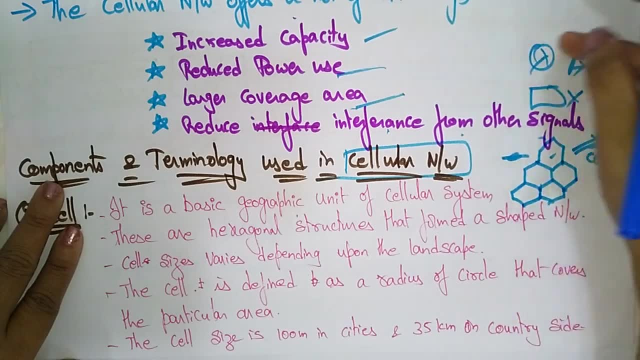 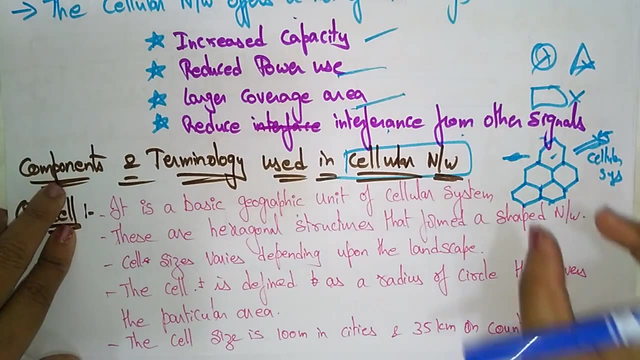 Why I am taking only the hexagonal? Because the hexagonal will cover the most area. The large covered area will be more in hexagonal when compared to the circle triangle and rectangle Means. it is compact, almost it is around 82%. it covers the area. 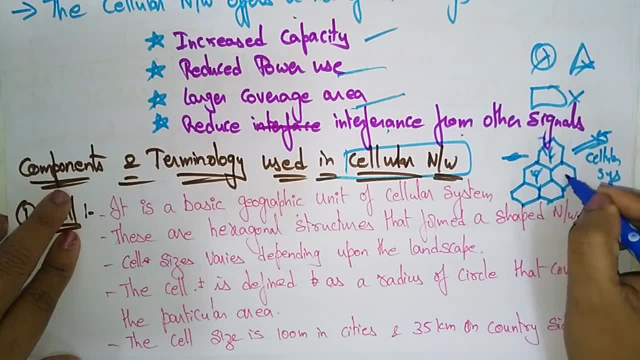 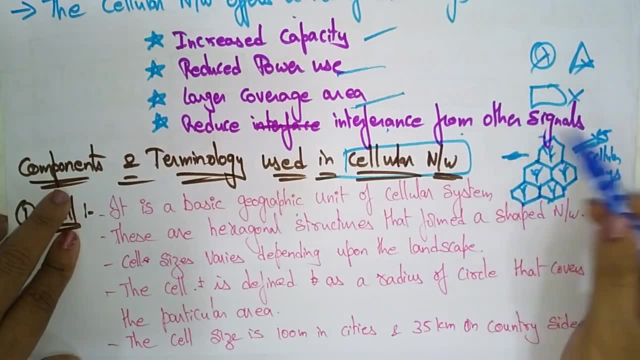 So whenever the tower is placed here, in each and every cell, every station, a tower is placed in each and every cell, it is the coverage area means. this signal how much area it will be covered. So if you take the hexagonal, it covers the large area. 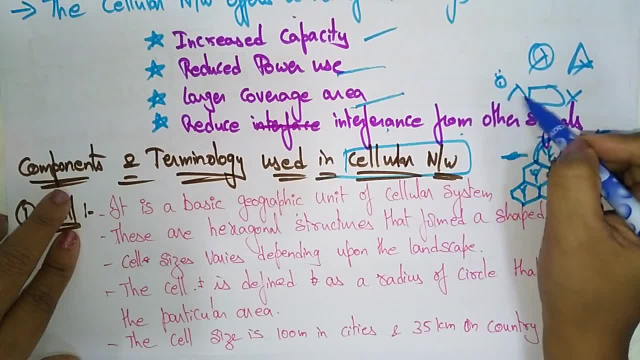 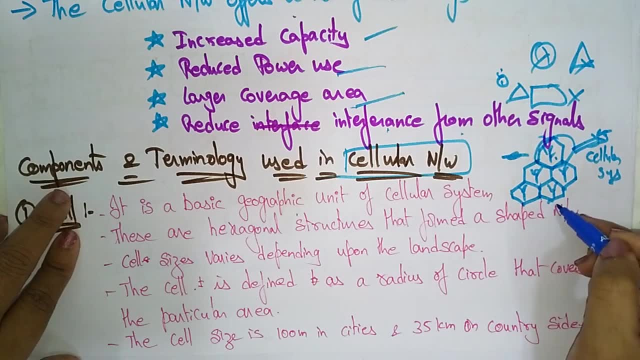 So if you take the circle, only the small area it will be covered. If you take the rectangle triangle, it covers only the less. So that's why they are taking the cell as a hexagonal. So it is a basic geographic unit of cellular system. 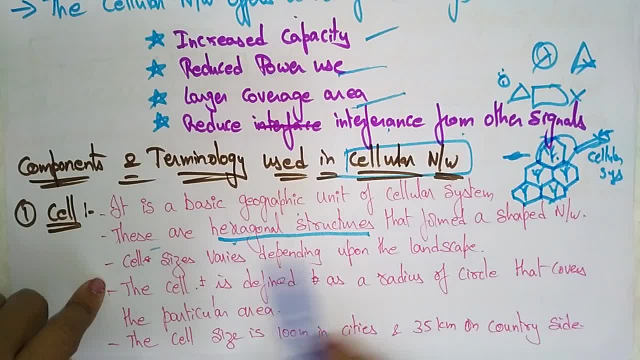 These are hexagonal structures that formed a shape network. Cell size varies depending upon the landscape- okay, how much landscape that it is having. the cell size will be vary Means how much tower that you are using, how much capacity of the tower is having. 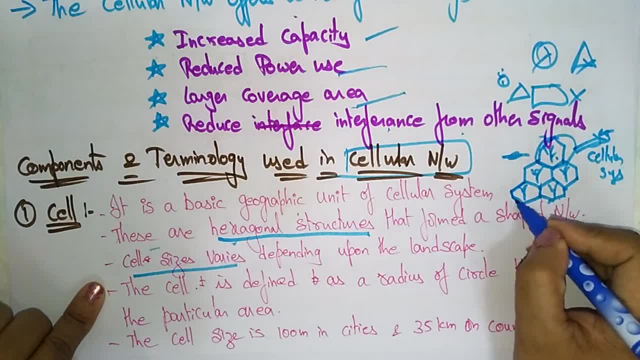 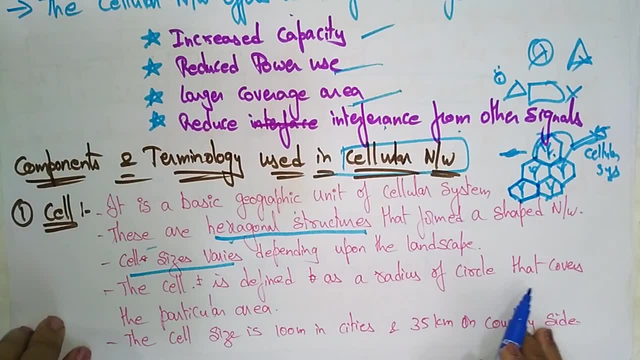 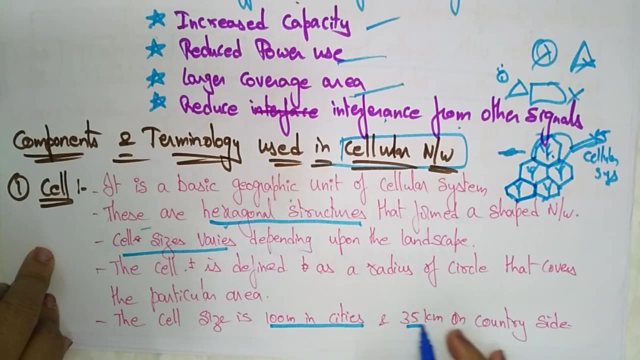 So, based on that, the cell size may be vary. So this is cell. okay, the cells are represented in the network. The cell is defined as a radius of a circle that covers a particular area. okay, The cell size is 100 meters in cities and 35 kilometers in the country side. 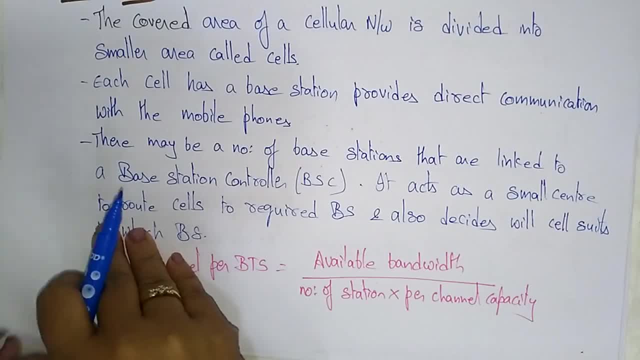 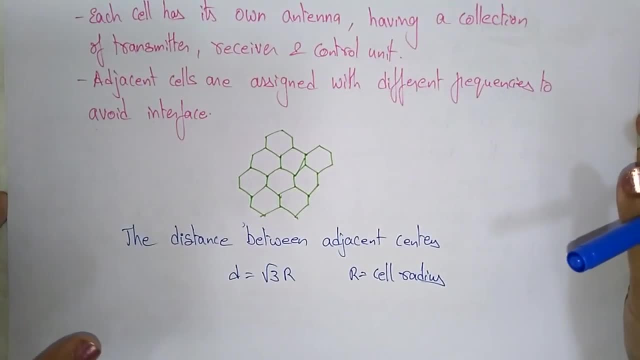 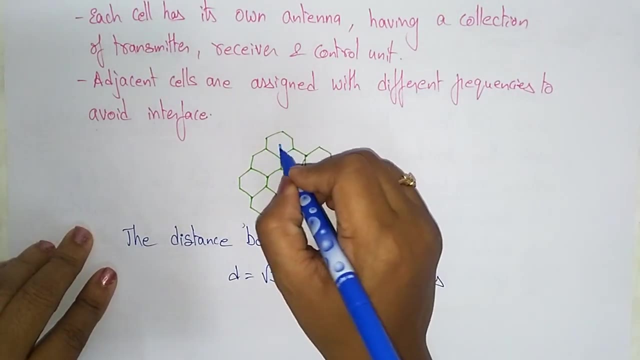 Now let's see this base station. What is this base station here? So, before that, I want to just show you this cell Here. each cell has its own antenna, having a collection of transmitter, receiver and the control unit. This is each cell. 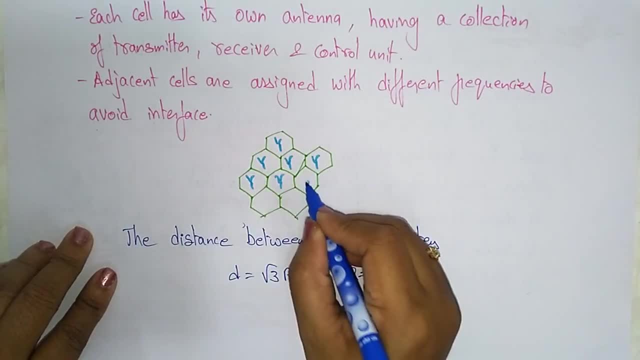 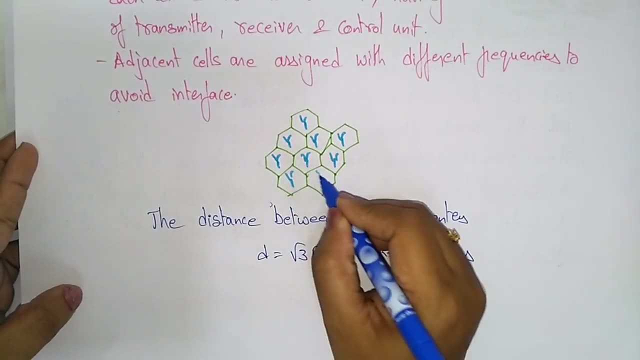 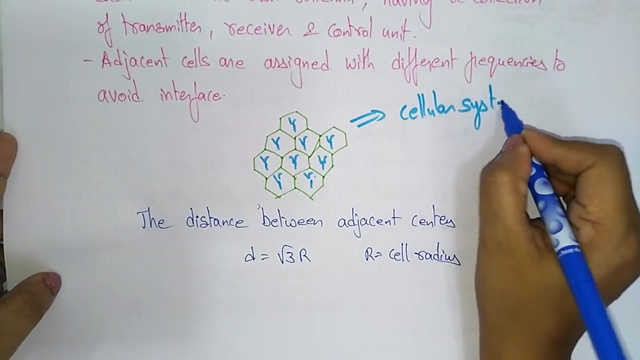 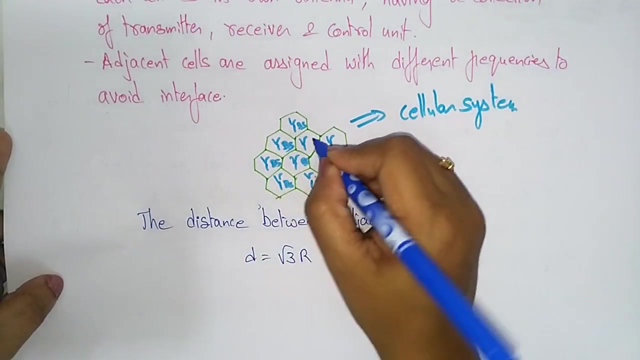 This is Just. I want to show you. this is a cell cellular system. you call it as a cellular system. In each cellular system you are having the base station, base station. okay, Now let me explain you this base station first. 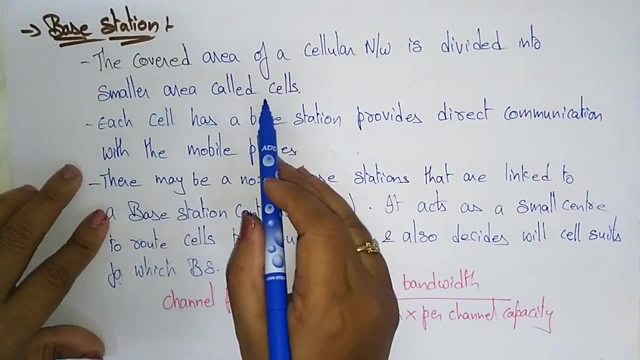 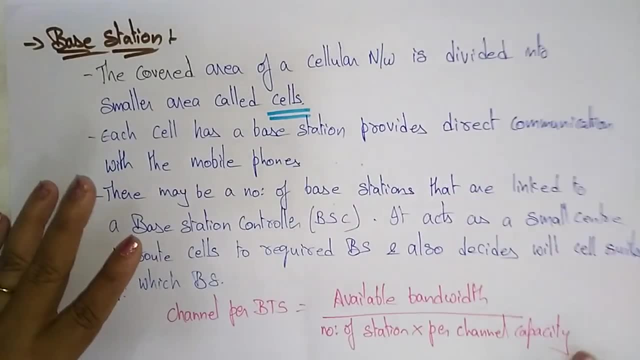 The covered area of a cellular network is divided Into smaller area, called cells, So that what I said each and every this hexagonal, you call it as a cell. So the covered area of a cellular network is divided into smaller area, called cells. 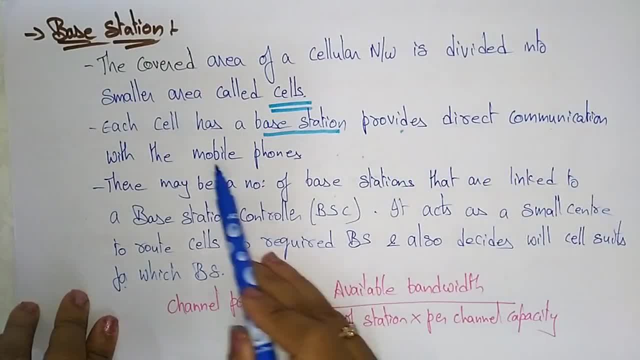 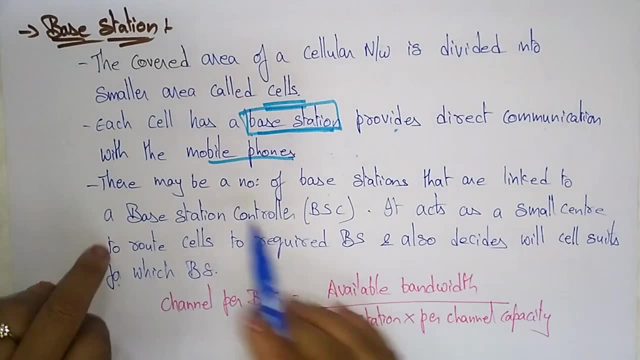 Each cell has a base station provided direct communication with the mobile phones. With the help of that base station only you are getting the direct communications okay with the mobile phones. There may be a number of base stations that are linked to the base station controller. 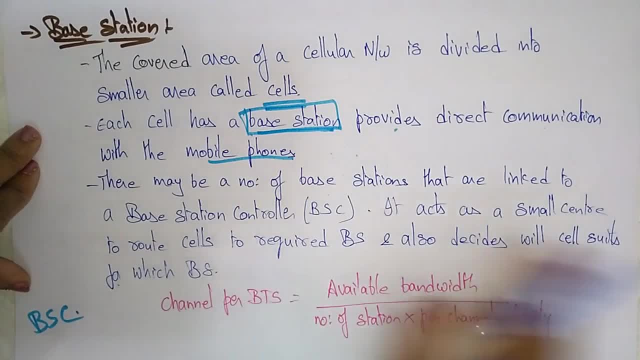 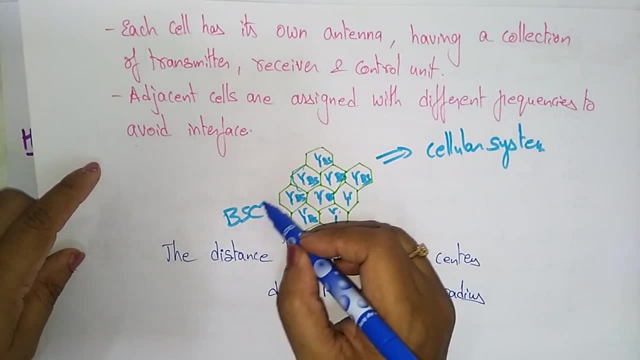 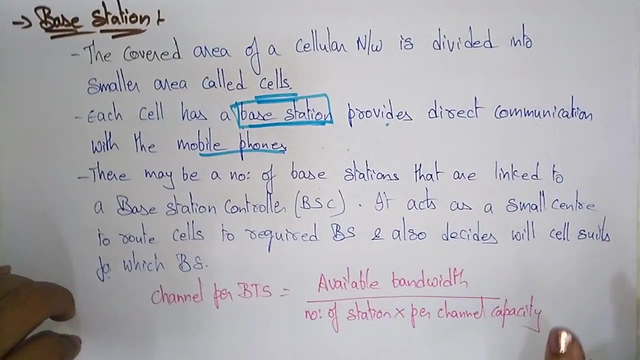 So a base station controller. This base station controller will be there. This base station controller is connecting so many number of. let's take somewhere around. the base station controller is there. This is going to monitor each and every cell. here Okay means not only a group of base stations which are nearer to that base station controller. 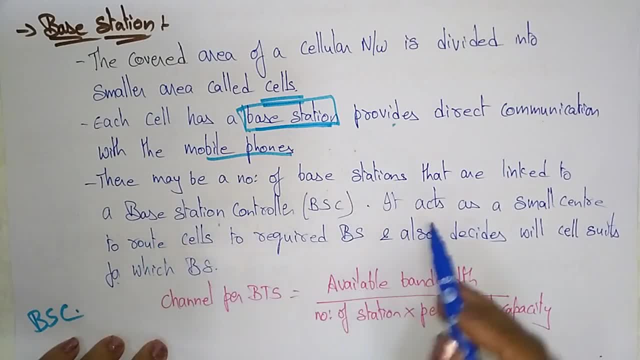 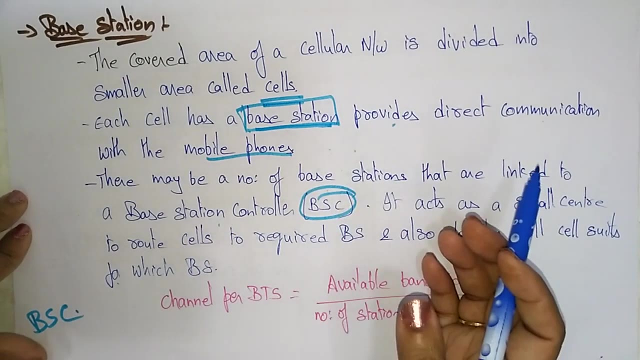 There may be a number of base stations that are linked to the base station controller. It acts as a small center to route cells to required base station And also decides will which cell suits for which base station. So this base station controller is deciding, whatever the signal that you are getting from the mobile phone. 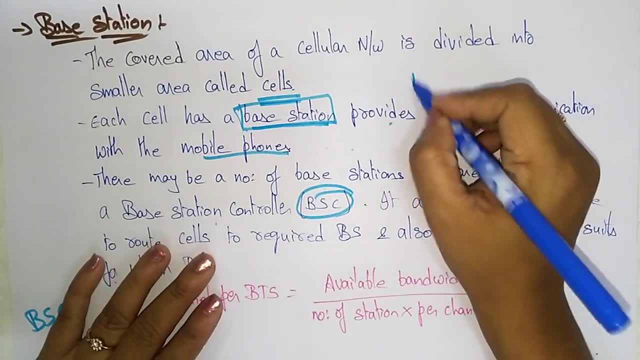 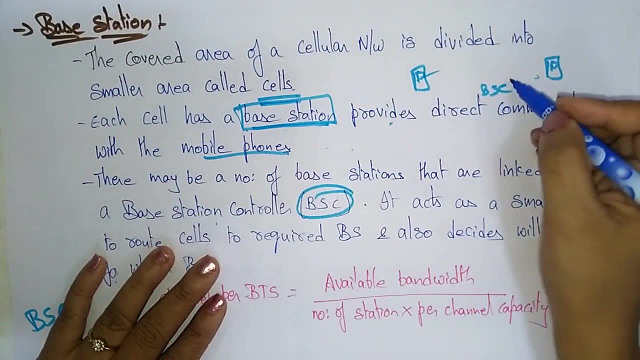 So that will be suit for which base station. So here one person is there, the mobile phone and another person is there They want to be communicated. So here the base station controller will be there and somewhere here a base station will be there. 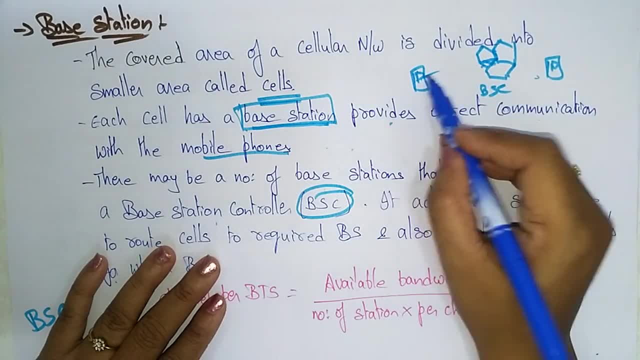 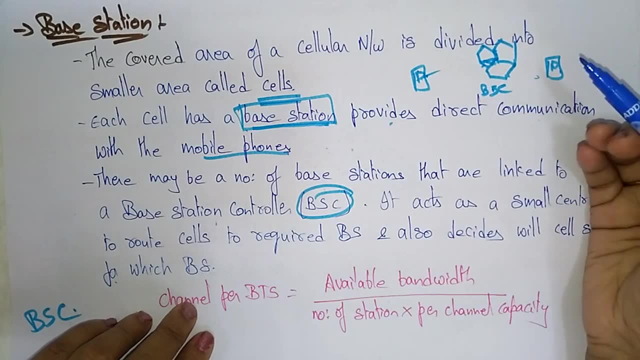 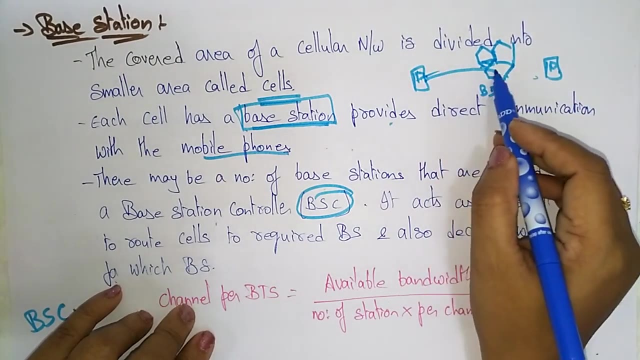 So if this person wants to communicate here, this base station controller decides which route to be required for the base station and also decides which cell suits for which base station. So it's just takes whatever that nearer to that and like this, communication will be established between the two persons. 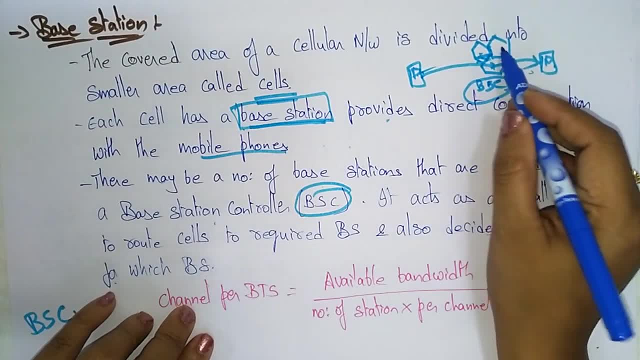 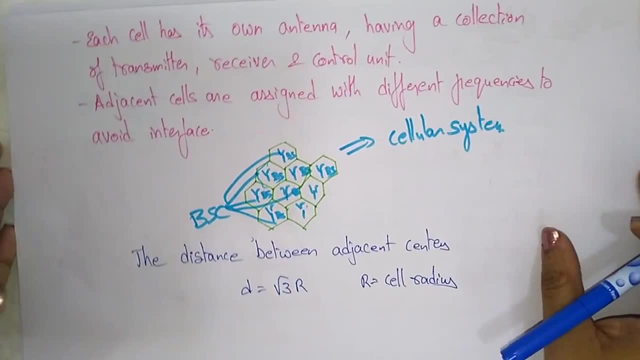 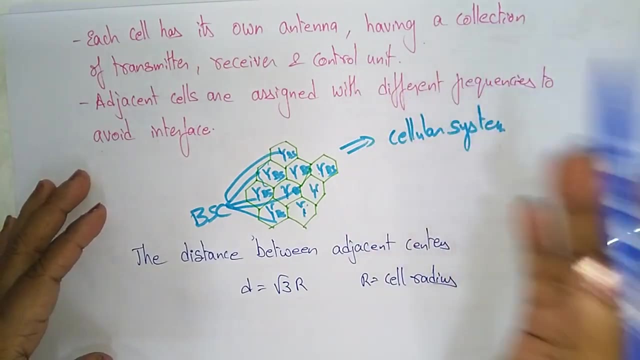 With the help of this base station controller. it is going to be monitor all the base stations. Each cell has its own antenna. So did you observe here, each cell is having their own antenna, Having a collection of transmitters, receivers and the control unit. 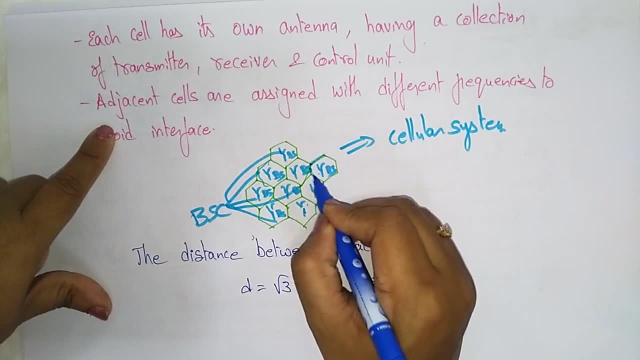 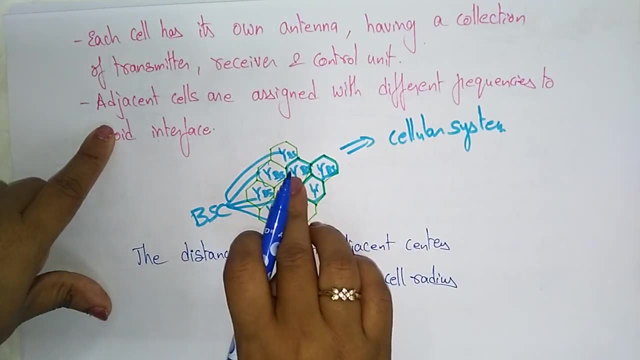 The adjacent cells are assigned. Did you observe here? all these are the. this is one cell. This is the adjacent cell to this cell and this is the adjacent cell to this cell. The adjacent cells are assigned with the different frequencies to avoid interface. 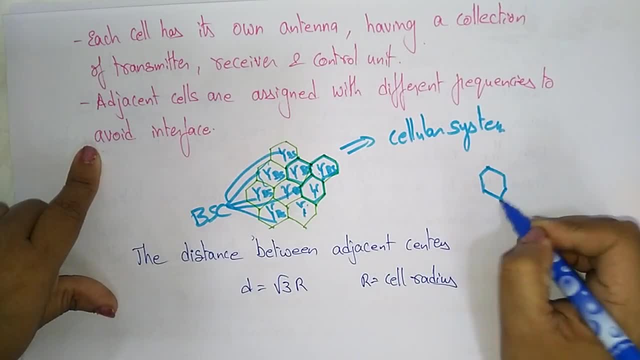 So observe that Whatever the cell that is having the adjacent cells, let's take this over the adjacent cells. This should be different frequency. Suppose this is 1 and take it as 2 and this is as 3.. These are the frequencies. 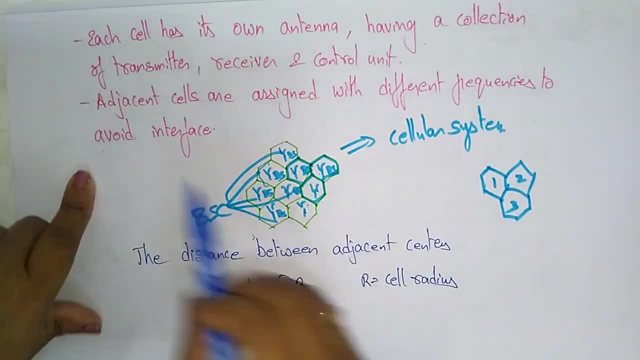 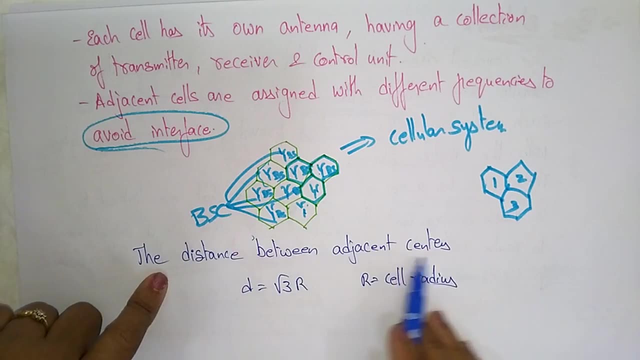 Adjacent cells are assigned with different frequencies to avoid the interface. To avoid interface, we have to use. they are using the different frequencies. The distance between the adjacent centers is: D, is equal to root 3, R, Where R is the cell radius. 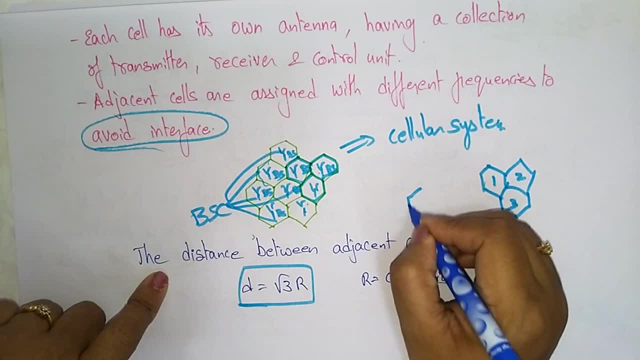 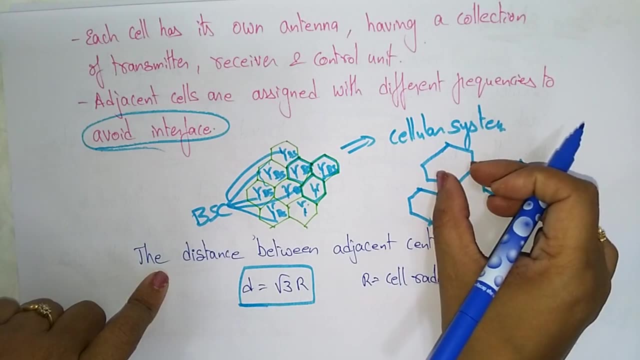 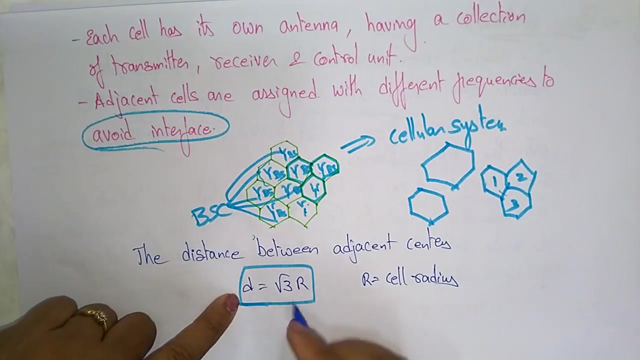 A cell radius means how much of size will be there. the radius Some cells is like big and some is small, So this is cell radius. The distance between the adjacent cells, adjacent centers, can be calculated by using: D is equal to root 3 R. 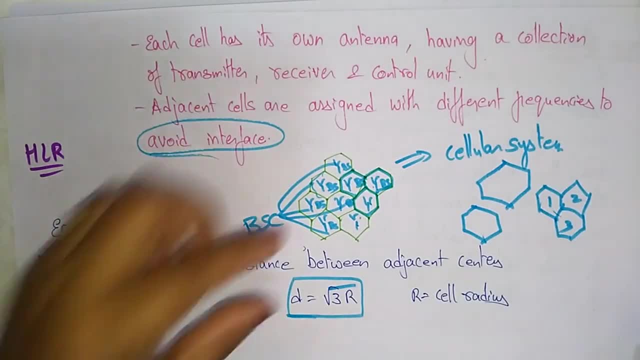 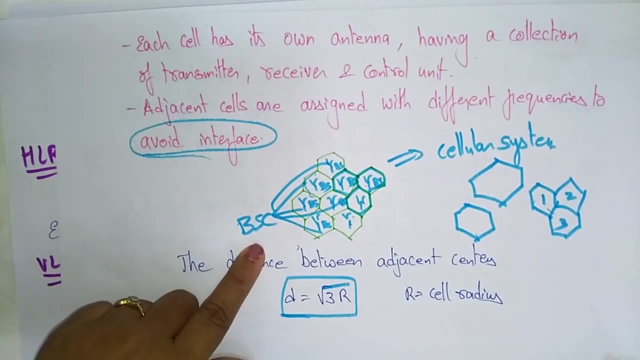 Okay, So these are the terminologies that we used in the cellular. This is a complete cellular network. In the cellular network, you learn what is a cell and what is a base station And what is a base station controller. Okay, 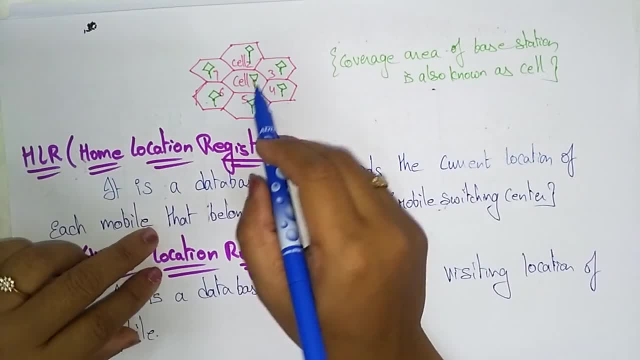 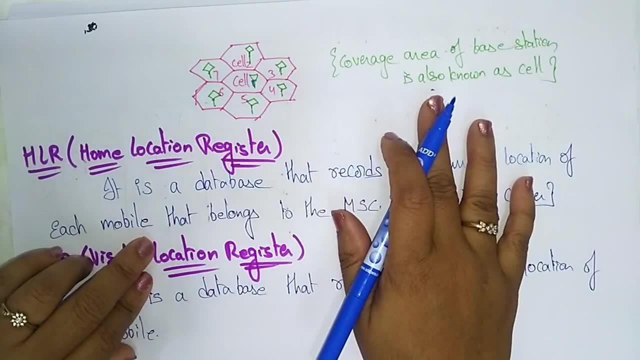 So here see the adjacent cells- is having the different frequencies: Cell 1,, 2,, 3,, 4,, 5,, 6,, 7.. So the coverage area of a base station is also known as a cell. 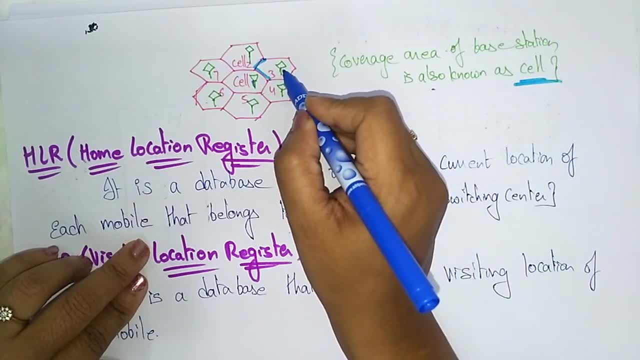 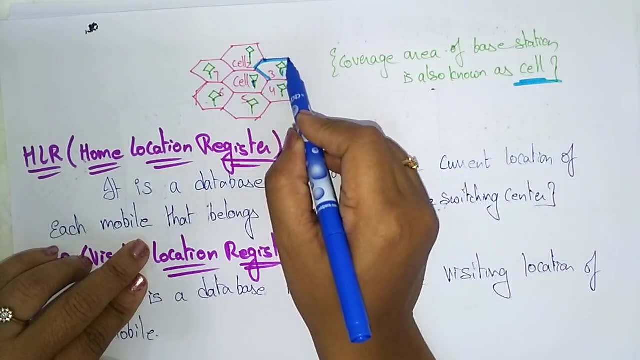 A base station coverage area, This base station, this is a base station And this is one base station for this cell. This is one base station for this cell. The coverage area of a base station- you call it as a cell. This base station covers only up to this cell only. 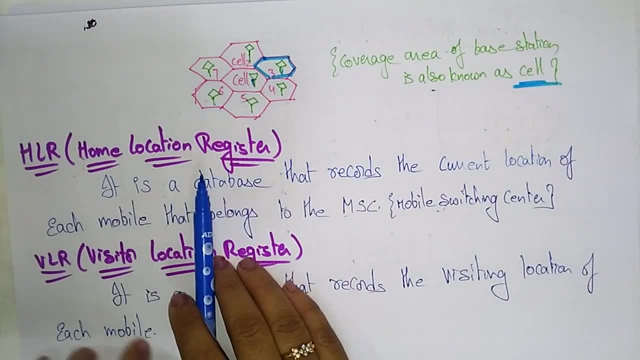 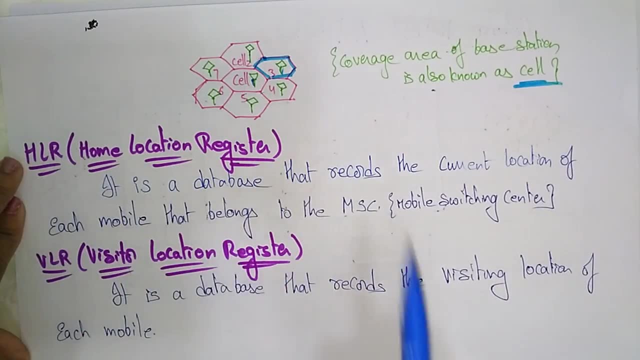 And another terminology that we used in the cellular concept, cellular network, is HLR- Home location register. It is a database- You call it as a database- that records the current location of each mobile that belongs to the mobile switching center. So here another term will be there. 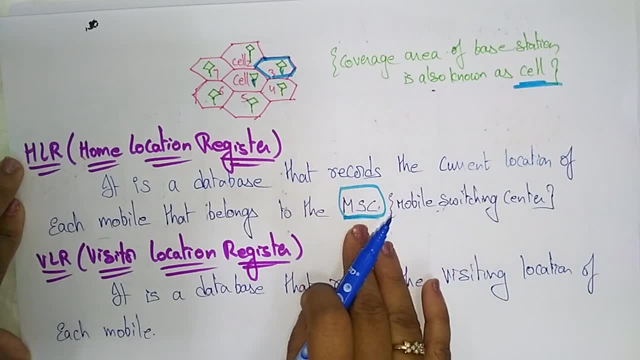 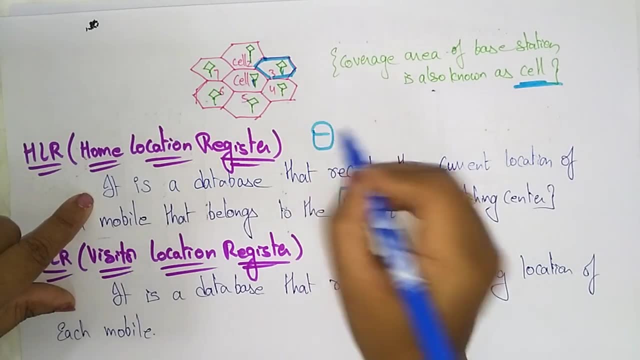 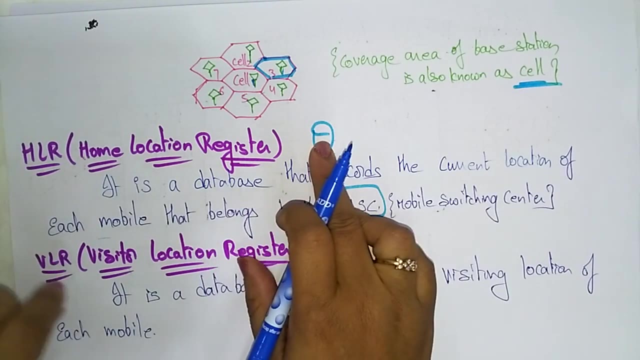 Not only the base station controller, the mobile switching center is there. So the Home location register is a database- You call it as a database- that records the current location, means at where you are present, records the current location of each mobile that belongs to the mobile switching center. 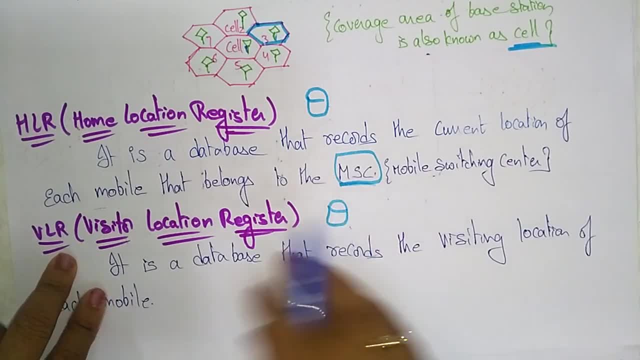 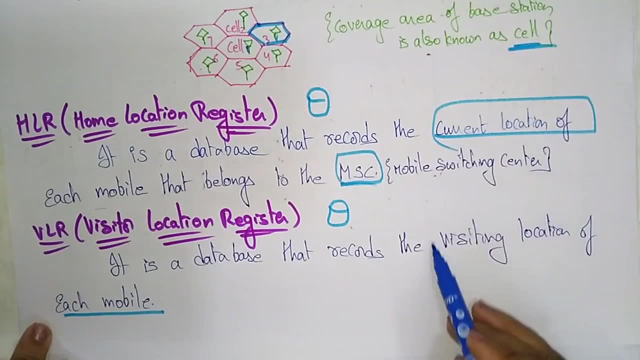 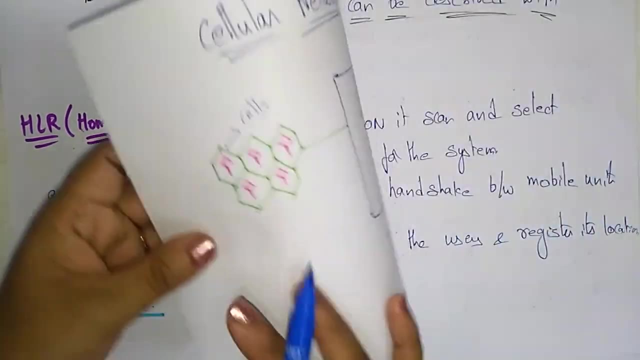 And VLR is also one database, visitor location register that records the visiting location of the each mobile. This is a current location and this is records the visiting location of each mobile. Okay, So, just these are the terminologies that we used in this cellular network. 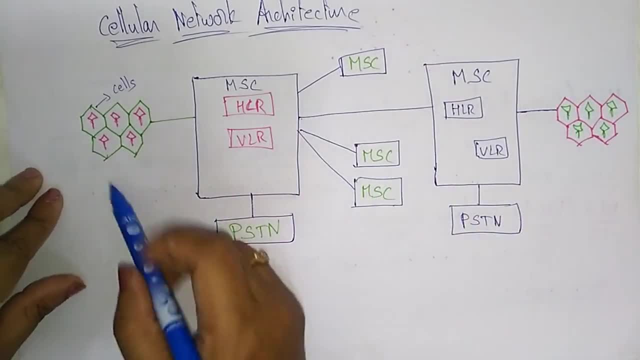 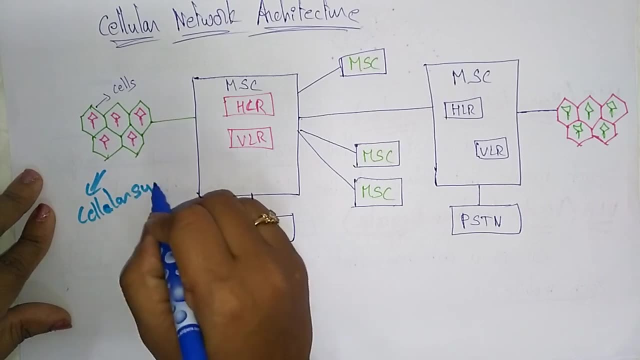 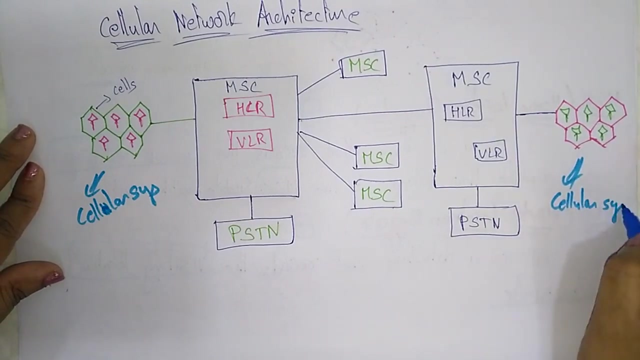 So here you can see the cellular network architecture. This is completely cellular system at one end Cellular system, Let's take from the receiver center, and it is another cellular system at the receiver side. Okay, Each having this, base stations are there. 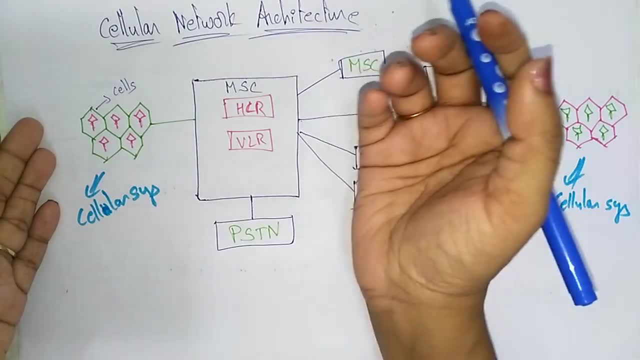 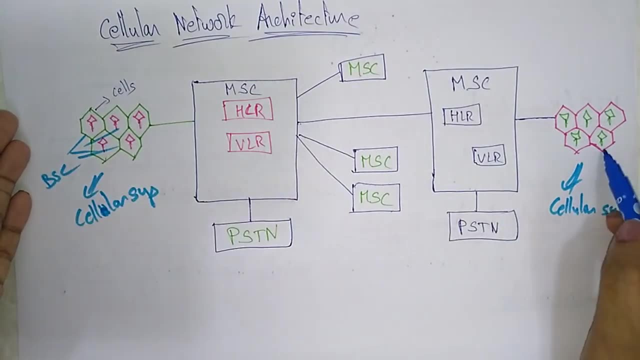 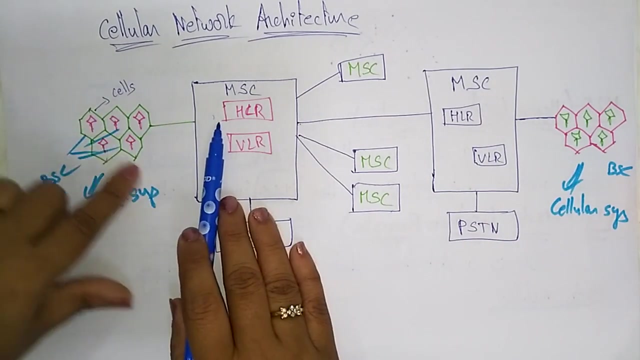 Each cell is having their own base station Which receives the transmitting the receives and transmitting the signals, and these are all controlled by the base station controller. So each cell, whatever the cell that is activating that base station, will sends to the message to the mobile switching controller. 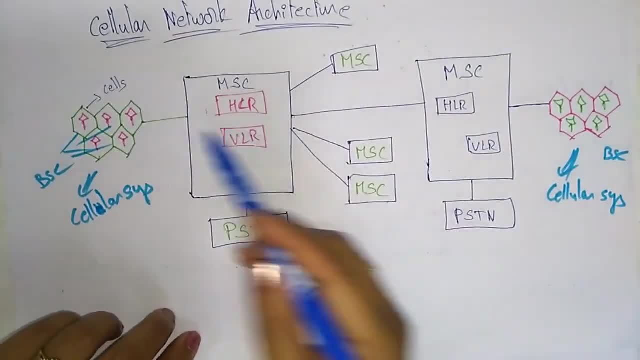 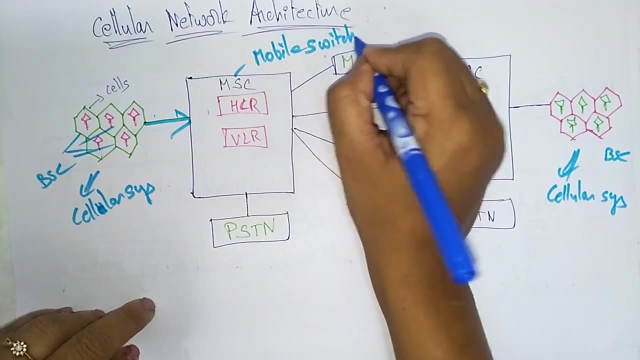 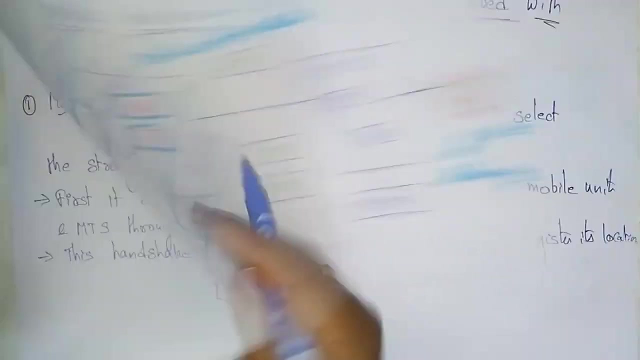 Okay, So MSC mobile switching center. So that will be sent to the mobile Switching center. So this mobile switching center is having the HLR and VLR. Okay, The HLR, I call it as a home location register. 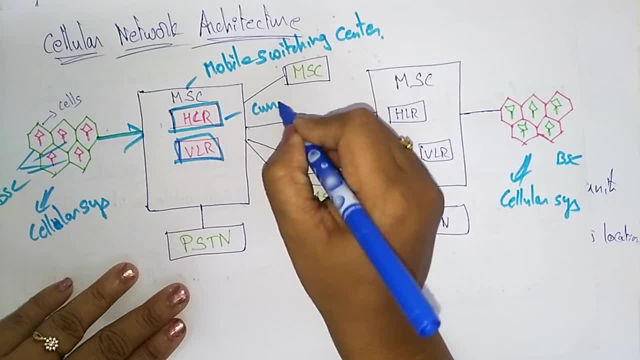 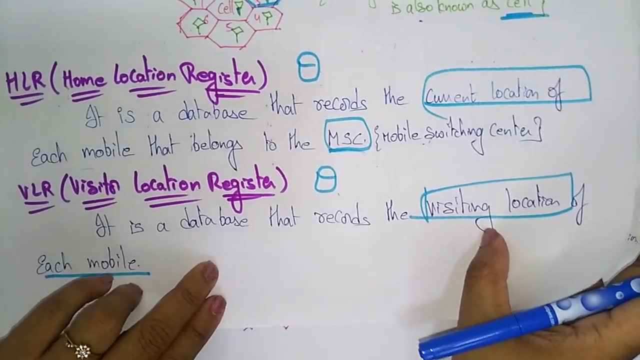 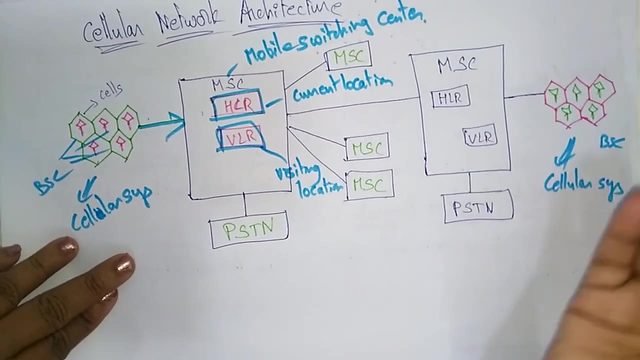 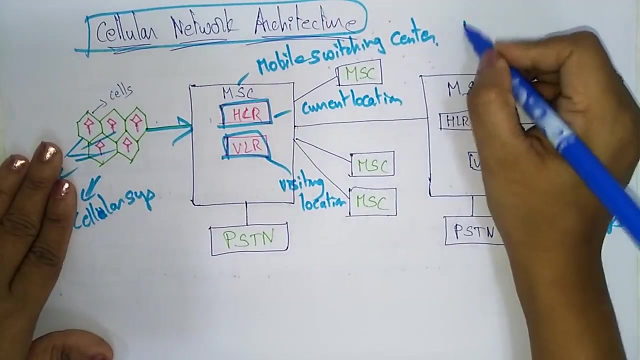 What it stores. It stores a current location. It stores the current location and VLR visitor location register. It stores a visiting location of mobile, Visiting location of mobile Means where that mobile is present, Actually the cellular network we used when we are moving from one place to another place. 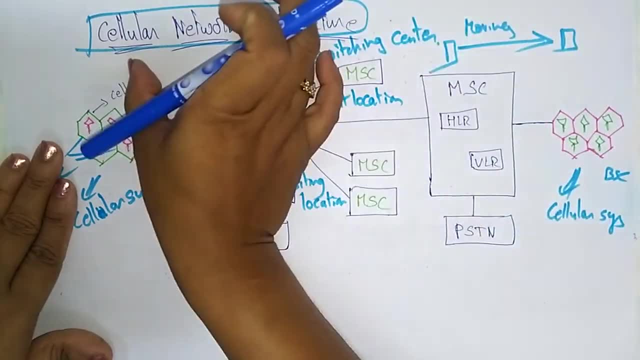 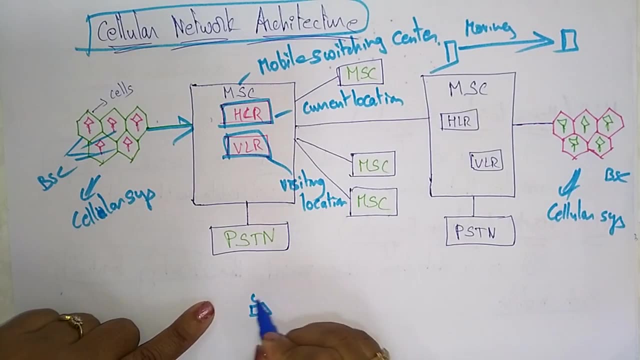 We are moving from one place to another place, So this cellular network will be active. So here how you are talking in the phone. Suppose you are at this place, Your car is at this place, You are moving. Okay, So whenever, while you are talking in the car, you are just talking in the car. 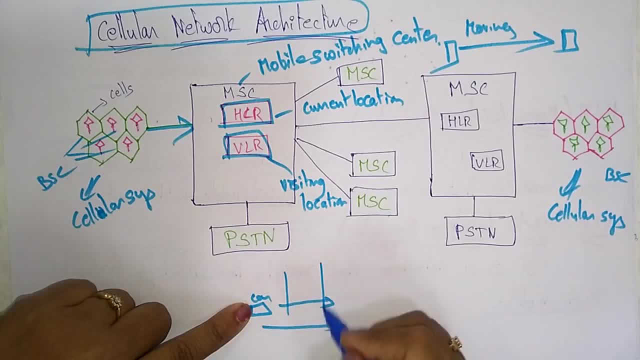 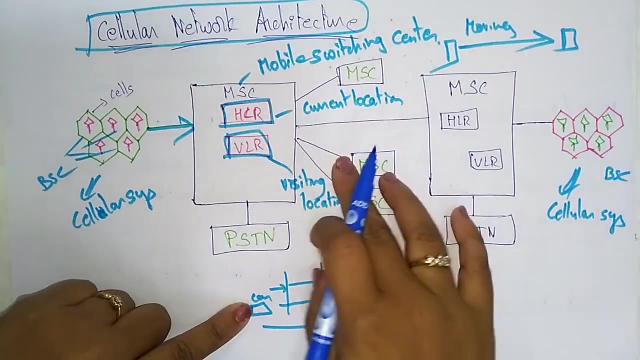 The car is moving this side, So whenever a different You are shipping this place to another place and this place to another place, The cellular network is able to manage your call without disconnecting. So how? With the help of this architecture. 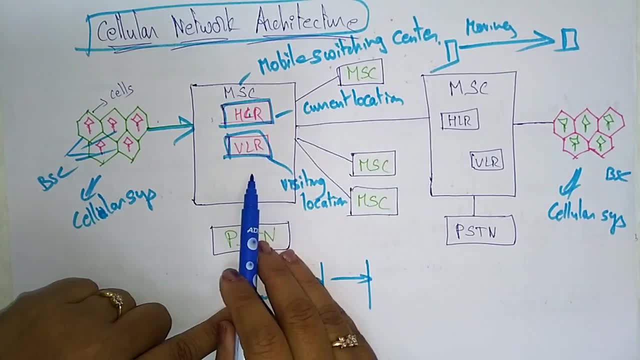 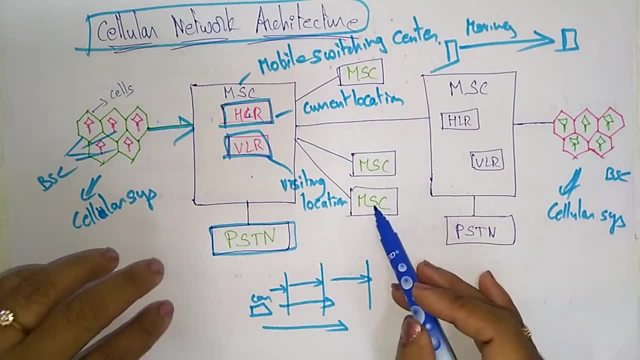 So here the mobile switching center holds the current location and the visiting location. Here the public's switching telephone network will be there, And this is also one mobile. So many mobile switching centers will be there. So, with the help of that mobile switching center, your call will be. 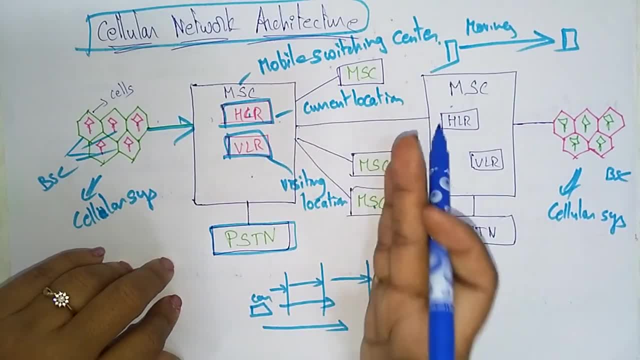 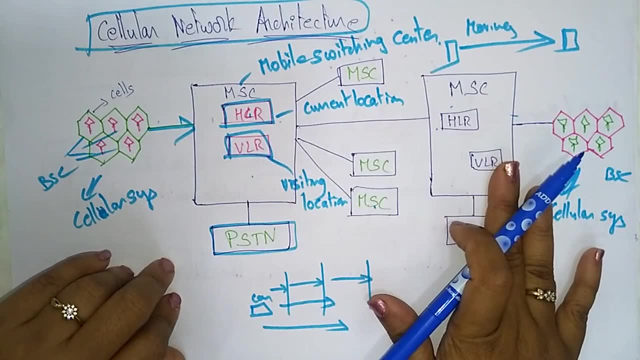 continue without disconnecting. Your call is continue without disconnecting. So, whenever you are moving, this will be shifting to this another mobile switching center And this will be shifting to another mobile servicing switching center. Okay, And the. finally it reaches your destination. 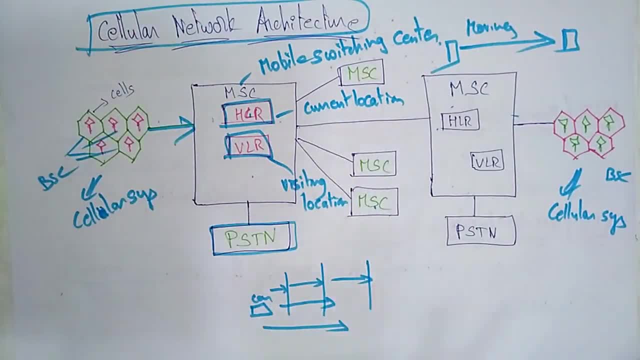 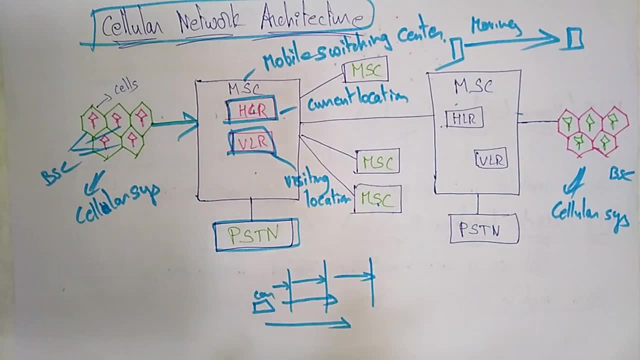 So, like that, the mobile switching center is holding everything information regarding your call and it is not help. It is helpful in not disconnecting your call. So this is about this. So basic terms that you are used in the cellular network architecture. Okay, Thank you.